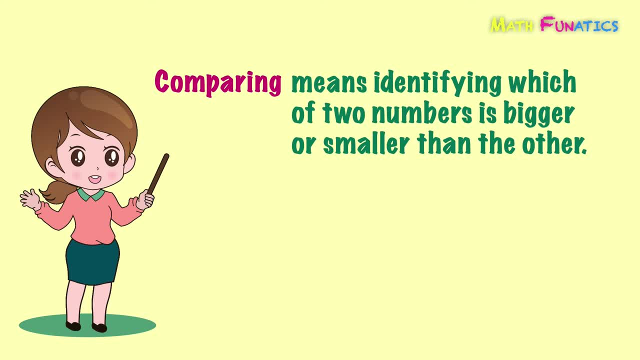 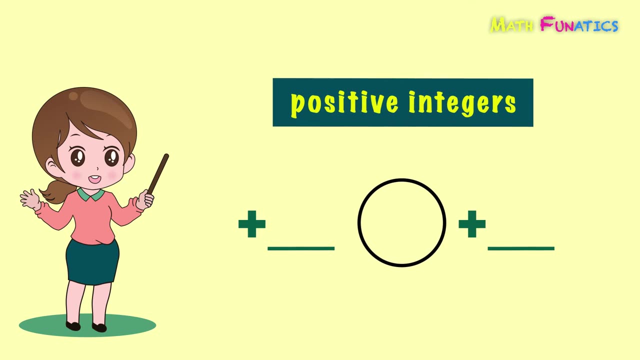 When comparing, we might also encounter numbers that are equal. Let us recall the symbols that we use in comparing. They are the greater than, less than and equal signs. When asked to compare positive integers, it is as simple as comparing whole numbers. 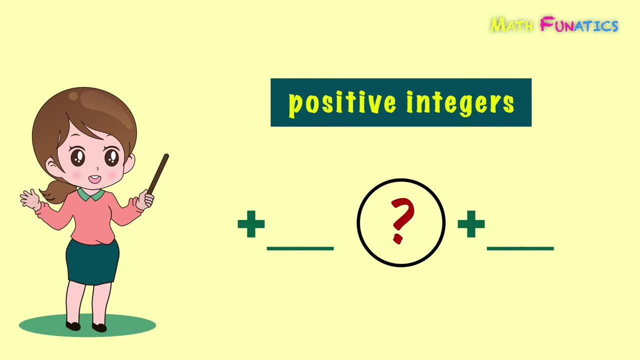 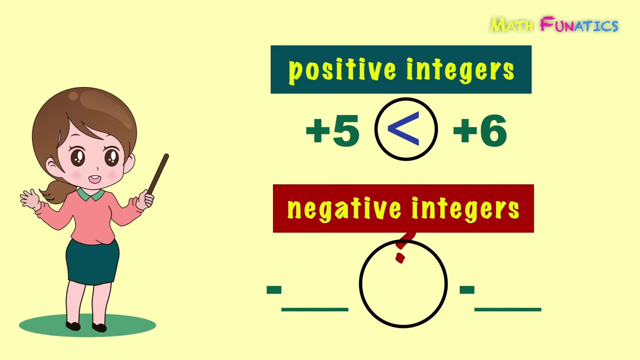 which we used to do during our early years in studying numbers. So if we compare positive 5 and positive 6, we know that 6 is bigger than 5.. But what if we are asked to compare two negative integers, say negative 5 and negative 6?? 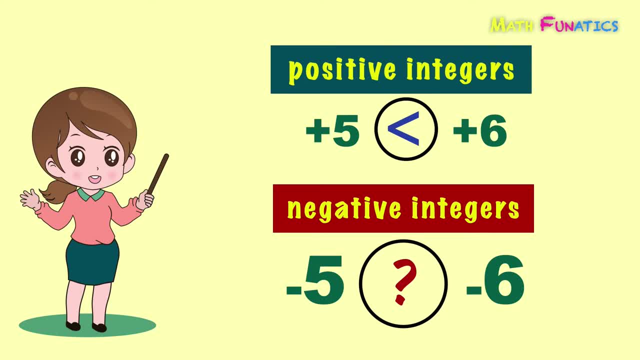 Which of the two negative integers is bigger? Is it negative 5 or negative 6?? Definitely, you might be wondering if we should apply the same way of comparison we did earlier with positive 5 and positive 6 to these two negative integers. 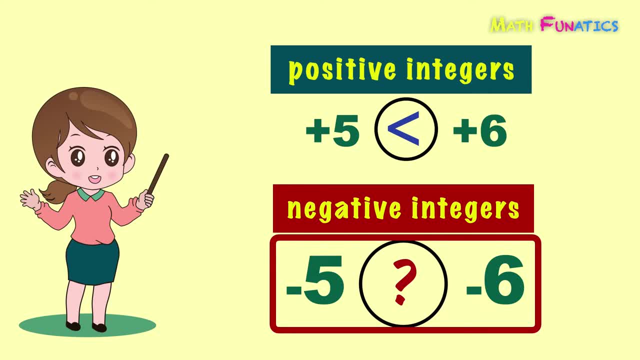 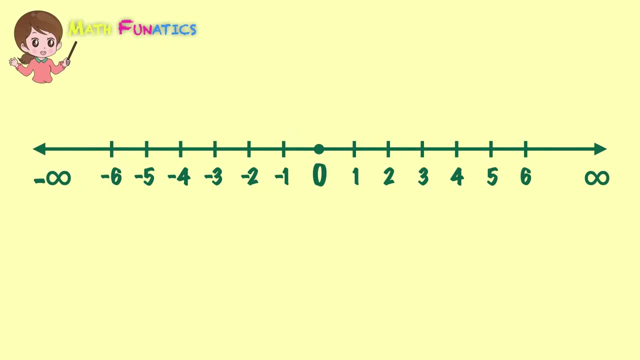 Let's see To have a better understanding. let us use a number line and see where these integers are located. With the number line, we need to remember that as the number goes from 0 to the right, the number gets bigger and bigger. 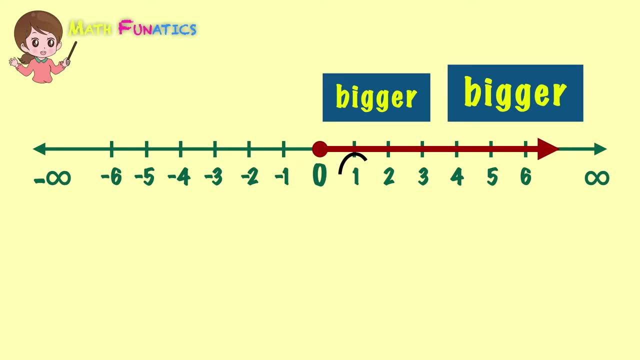 and bigger. That is why 1 is greater than 0,, 2 is greater than 1, and, with our example earlier, 6 is greater than 5.. How about if we go the other way around, to the opposite direction? 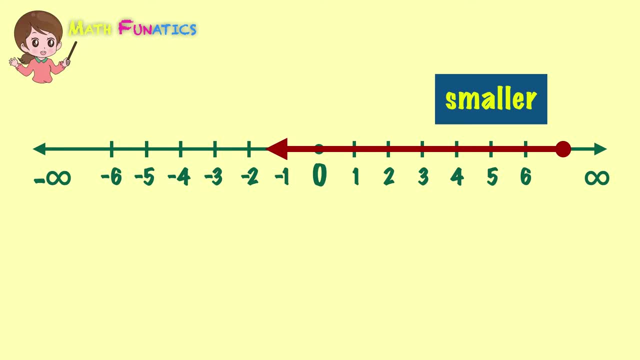 As the number goes to the left, the number gets smaller and smaller. That's why 0 is less than 1,, 1 is less than 2, and, with our example earlier, 5 is less than 6.. The same rules apply as we extend the number line. 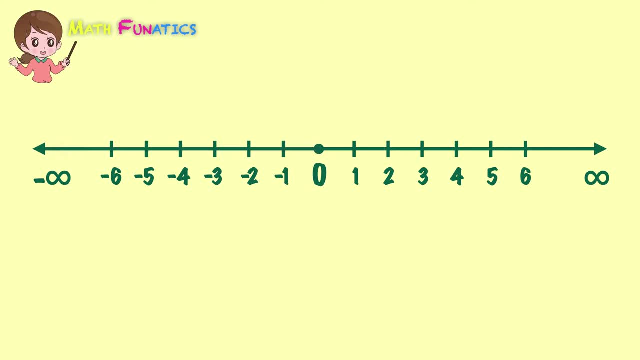 and deal with the negative numbers. Again, the numbers get bigger as you go to the right and smaller as you go to the left. So locating the two negative integers that were given in our question earlier- negative 5 and negative 6,. 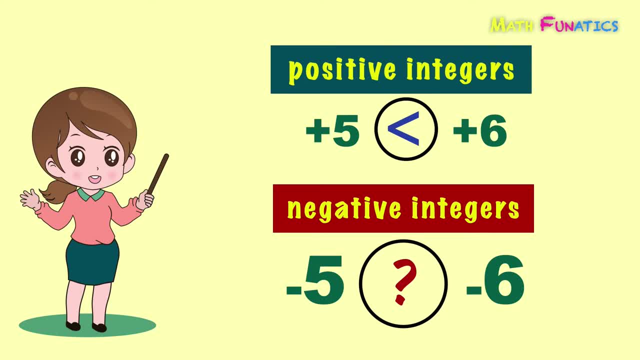 Which of the two negative integers is bigger? Is it negative 5 or negative 6?? Definitely, you might be wondering if we should apply the same way of comparison we did earlier with positive 5 and positive 6 to these two negative integers. 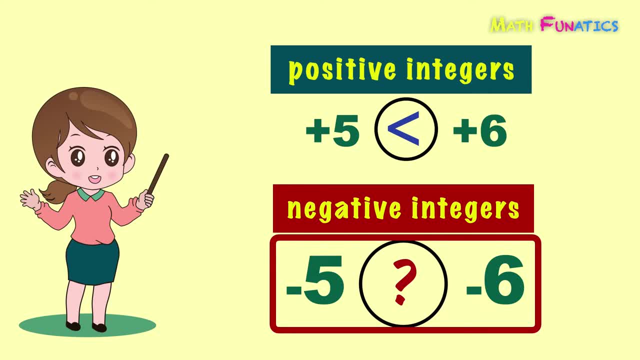 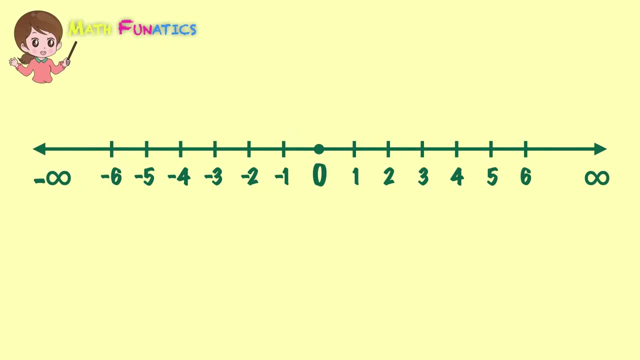 Let's see To have a better understanding. let us use a number line and see where these integers are located. With the number line, we need to remember that as the number goes from 0 to the right, the number gets bigger and bigger. 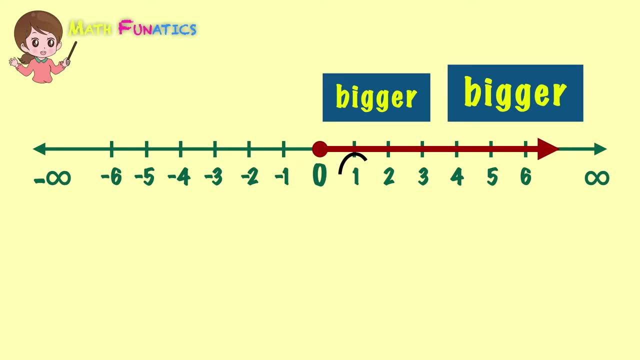 and bigger. That is why 1 is greater than 0,, 2 is greater than 1, and, with our example earlier, 6 is greater than 5.. How about if we go the other way around, to the opposite direction? 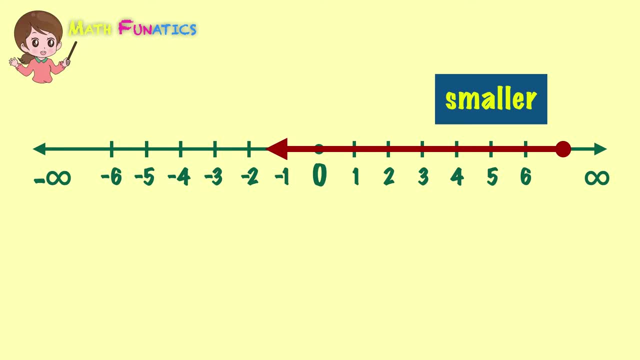 As the number goes to the left, the number gets smaller and smaller. That's why 0 is less than 1,, 1 is less than 2, and, with our example earlier, 5 is less than 6.. The same rules apply as we extend the number line. 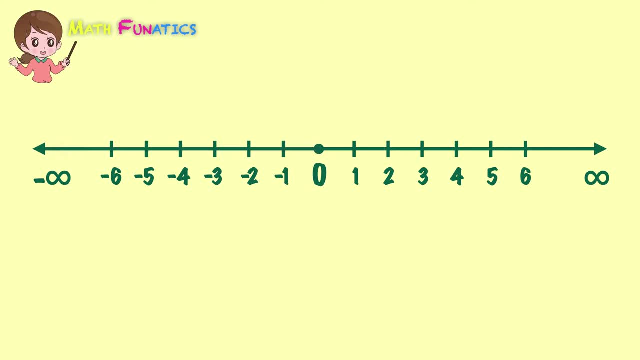 and deal with the negative numbers. Again, the numbers get bigger as you go to the right and smaller as you go to the left. So locating the two negative integers that were given in our question earlier- negative 5 and negative 6,. 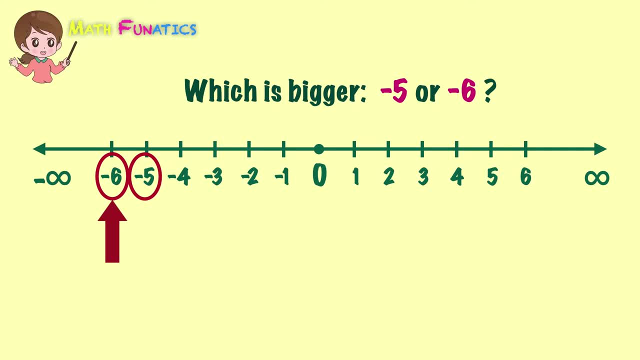 we see that negative 6 is on the left of negative 5.. Therefore, we can conclude that it is negative 5 that is bigger between negative 5 and negative 6.. So we do not base the comparison of negative 5 and negative 6. 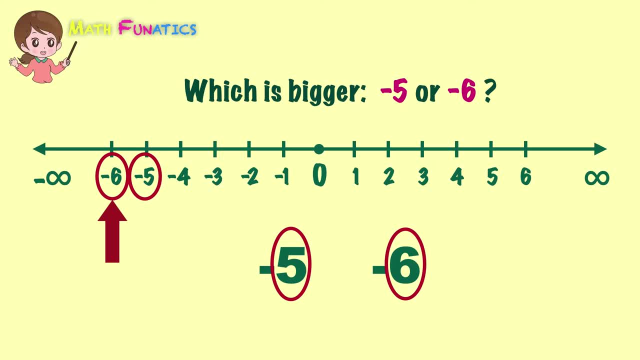 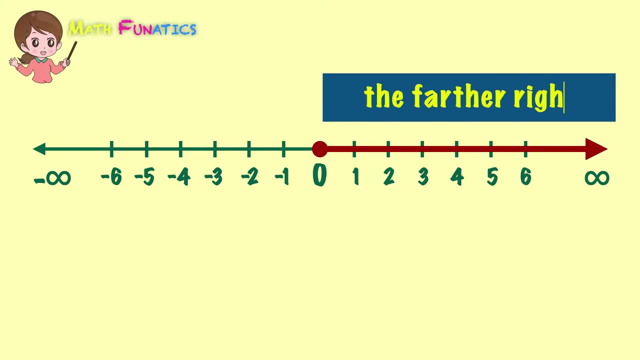 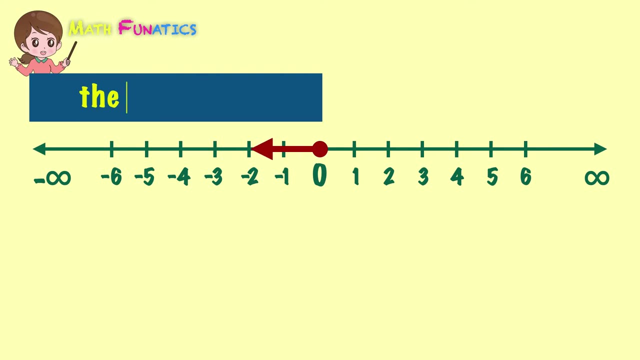 just by the number that appears with the sign. To let you further understand the concept of comparing integers: the farther the number on the positive side of the number line, the greater the value is, The farther the number on the negative side of the number line. 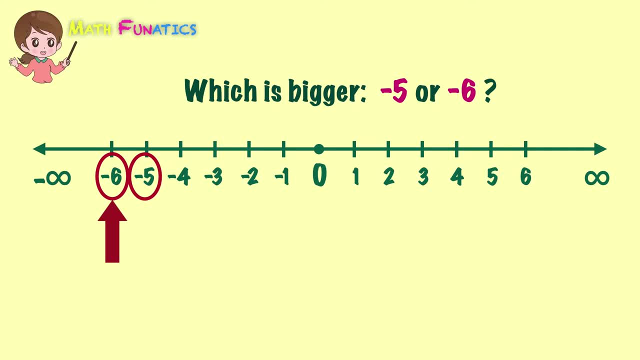 we see that negative 6 is on the left of negative 5.. Therefore, we can conclude that it is negative 5 that is bigger between negative 5 and negative 6.. So we do not base the comparison of negative 5 and negative 6. 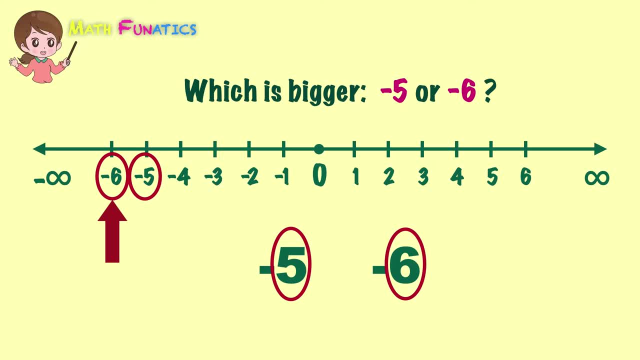 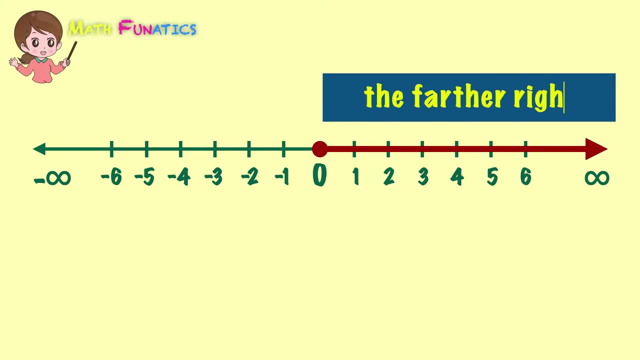 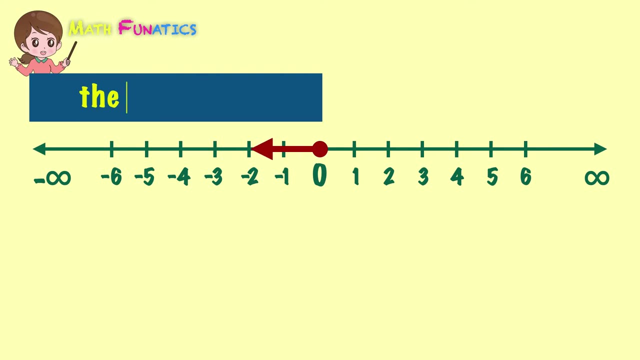 just by the number that appears with the sign. To let you further understand the concept of comparing integers: the farther the number on the positive side of the number line, the greater the value is, The farther the number on the negative side of the number line. 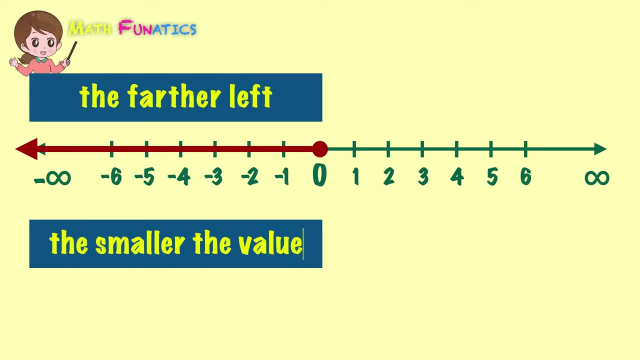 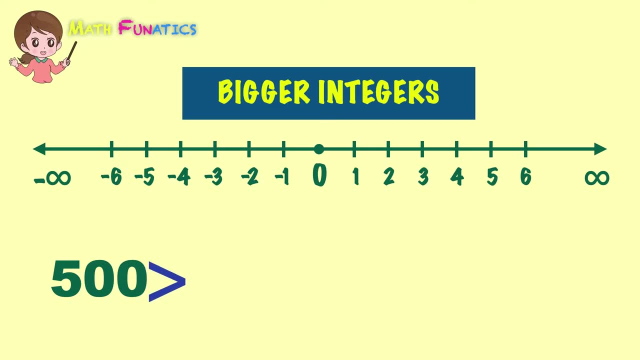 the smaller the value is. This is very applicable when dealing with bigger integers. So positive 500 is greater than positive 50, and negative 500 is less than negative 50.. Going back to the basics of a number line, positive integers are on the right of 0. 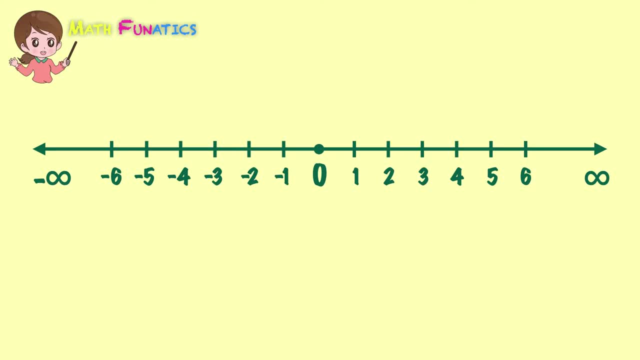 and negative integers are on the left of 0.. From this we can conclude that all positive integers are greater than 0 and all negative integers are less than 0.. Let's have some concrete examples. Lani, Lisa and Linda went to the cafeteria to take their snacks. 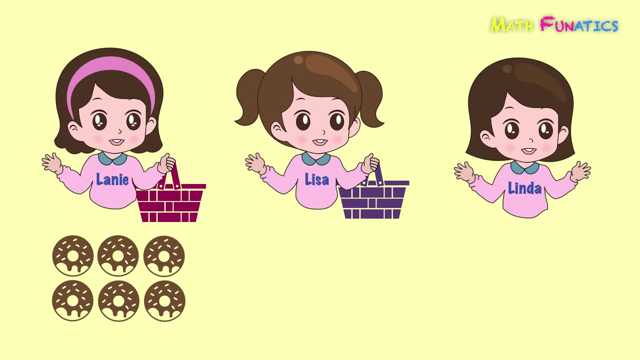 Lani brought six doughnuts. Lisa, on the other hand, brought two doughnuts. Unfortunately, Linda forgot to bring her snacks for the day, So Lani decided to give her two doughnuts, which Linda promised to pay the next day. 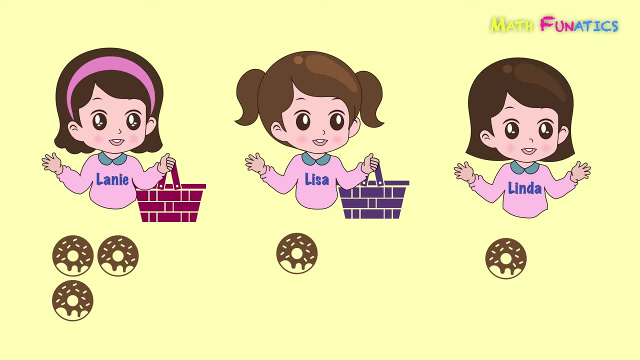 Each of the girls ate two doughnuts for their snacks. After their snacks, Lani still has two extra doughnuts left, which we write as positive 2.. Lisa has no more doughnuts left, so we write it as 0.. And Linda owes Lani two doughnuts. 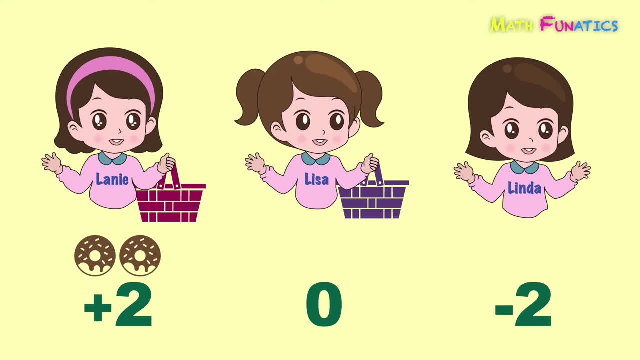 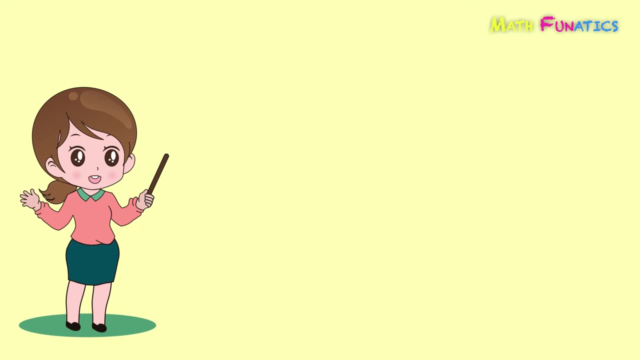 which we write as negative 2.. We can now see from here that negative integers such as negative 2,, which is our representation for Linda's case, is less than 0.. Now we're done comparing two positive integers, two negative integers. 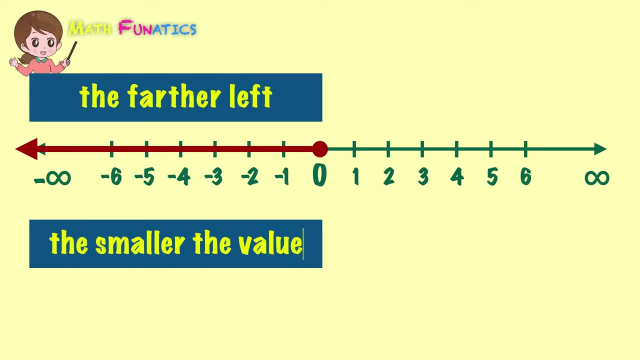 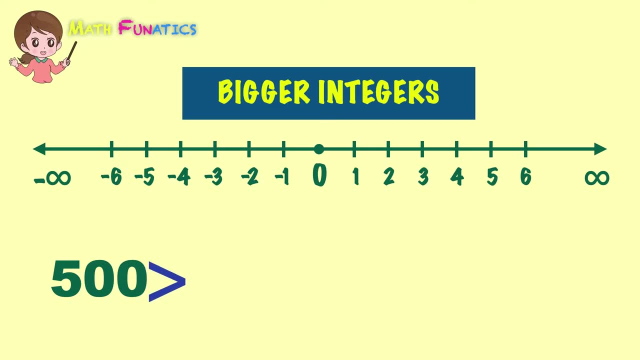 the smaller the value is. This is very applicable when dealing with bigger integers. So positive 500 is greater than positive 50, and negative 500 is less than negative 50.. Going back to the basics of a number line, positive integers are on the right of 0. 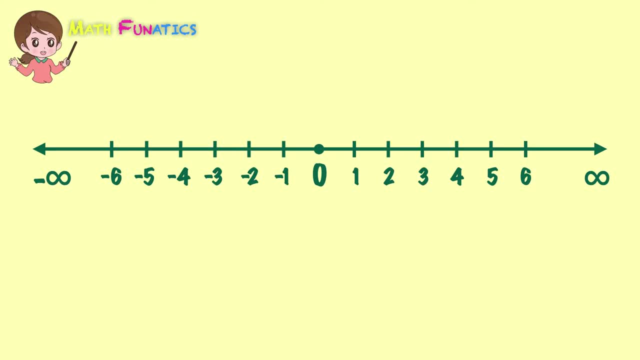 and negative integers are on the left of 0.. From this we can conclude that all positive integers are greater than 0 and all negative integers are less than 0.. Let's have some concrete examples. Lani, Lisa and Linda went to the cafeteria to take their snacks. 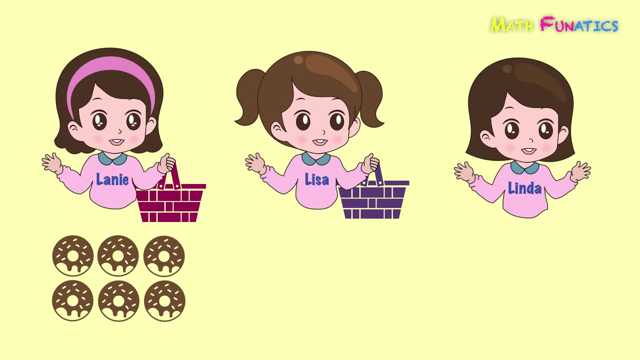 Lani brought six doughnuts. Lisa, on the other hand, brought two doughnuts. Unfortunately, Linda forgot to bring her snacks for the day, So Lani decided to give her two doughnuts, which Linda promised to pay the next day. 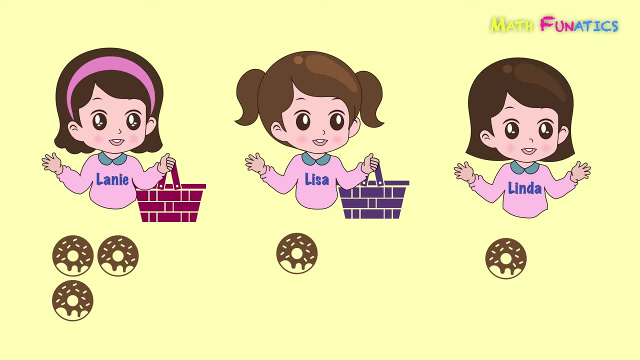 Each of the girls ate two doughnuts for their snacks. After their snacks, Lani still has two extra doughnuts left, which we write as positive 2.. Lisa has no more doughnuts left, so we write it as 0.. And Linda owes Lani two doughnuts. 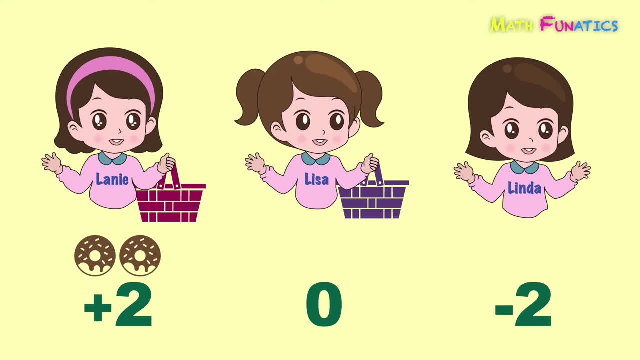 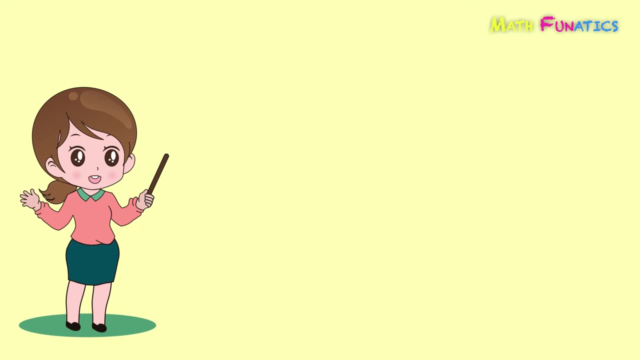 which we write as negative 2.. We can now see from here that negative integers such as negative 2,, which is our representation for Linda's case, is less than 0.. Now we're done comparing two positive integers, two negative integers. 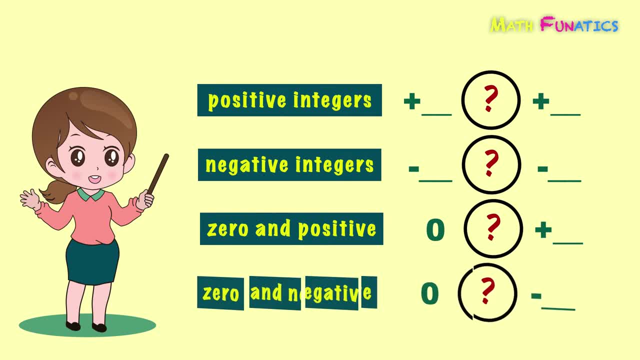 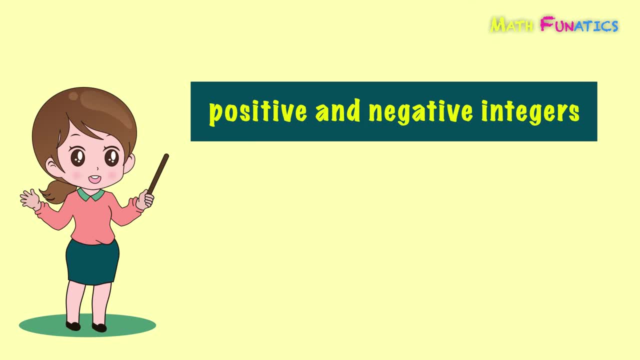 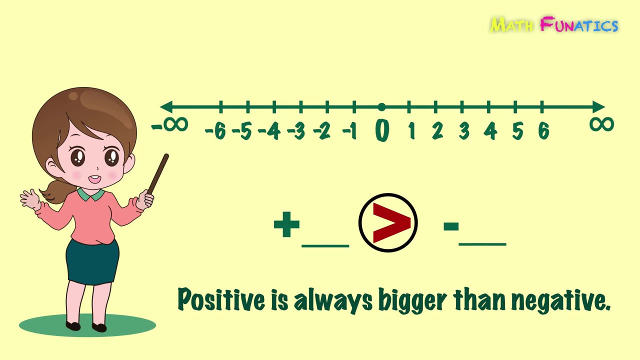 zero and positive integers and zero and negative integers. How about positive and negative integers? This is actually the easiest. It's because a positive number is always bigger than a negative number. We can see right away on the number line that all the positive numbers are on the right side of the number line. 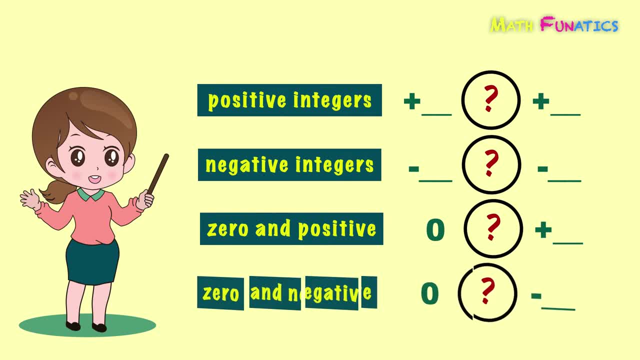 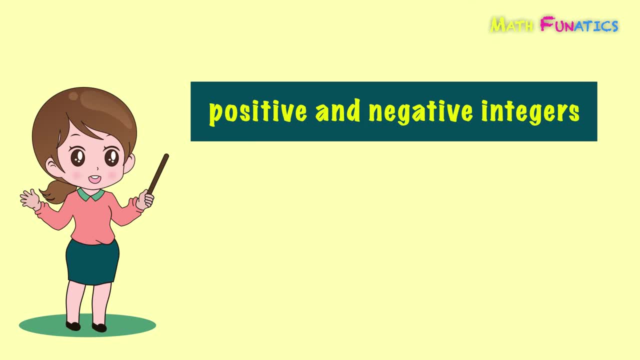 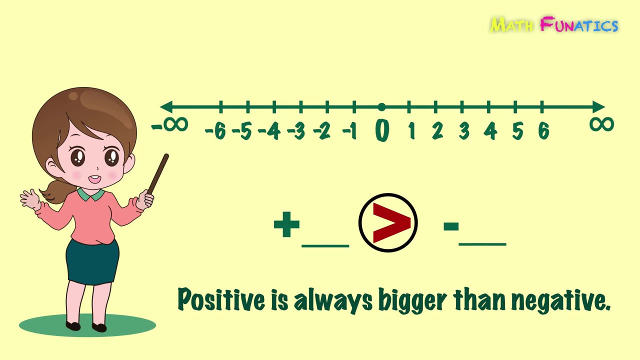 zero and positive integers and zero and negative integers. How about positive and negative integers? This is actually the easiest. It's because a positive number is always bigger than a negative number. We can see right away on the number line that all the positive numbers are on the right side of the number line. 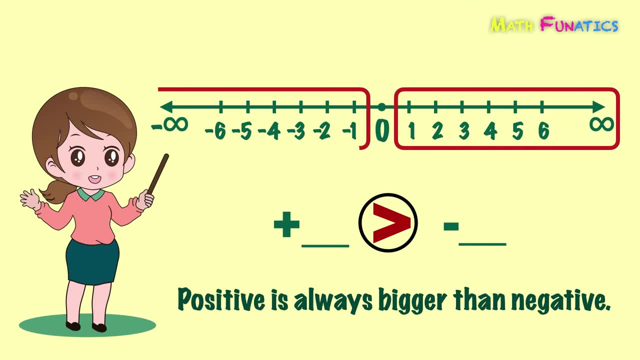 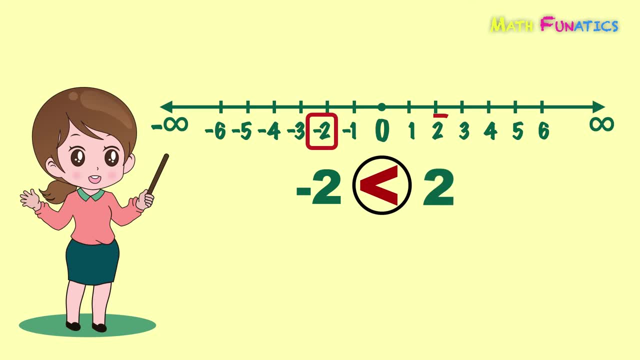 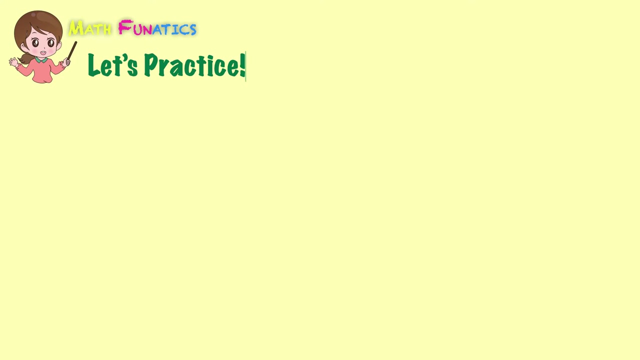 And all the negative numbers are on the left. So negative 2 is less than 2.. Negative 6 is less than 6.. Negative 100 is less than 100.. Now let's practice what you've learned about comparing integers. 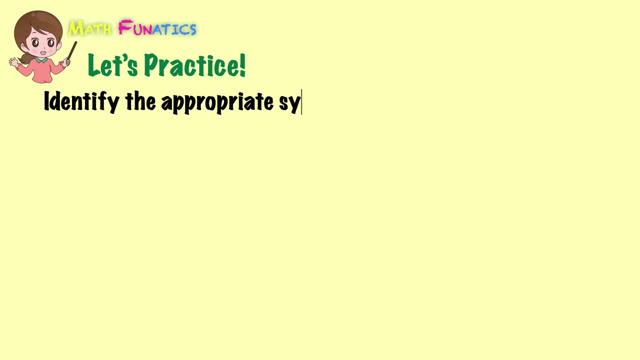 Identify the appropriate symbol for each comparison. The first is positive 18 and positive 11.. Since both are positive and 18 is on the right of 11 in the number line, then 18 is greater than 11.. Next we have positive 50 and 50.. 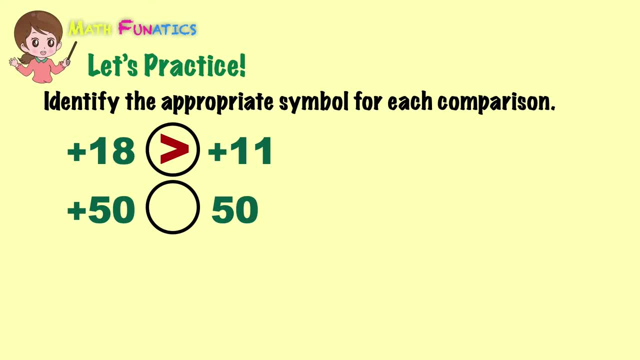 Both are actually positive 50, even though the second number has no sign. So they are equal: Negative 45 and negative 50, both are negative integers. Negative 45 is on the right of negative 54 and in fact nearer to zero. 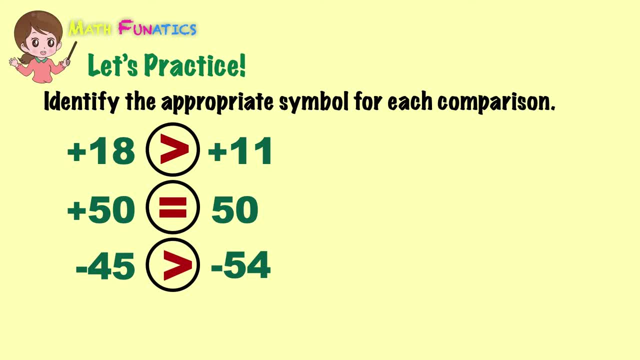 So negative 45 is greater than negative 54.. Negative 600 and negative 60. Negative 600 looks quite bigger than negative 60, but then it is actually found on the far left side of negative 60. So negative 600 is less than negative 60.. 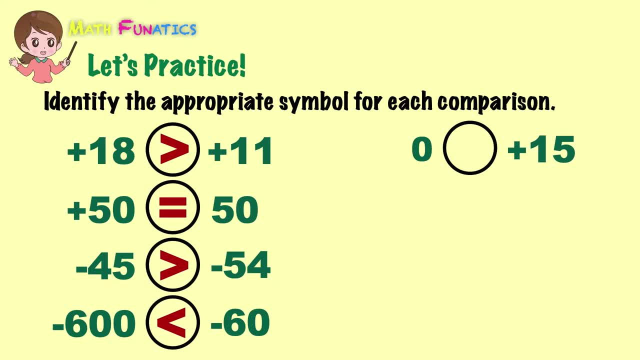 Zero and positive 15.. We've mentioned earlier that all positive numbers are greater than zero. So zero is less than 15.. Zero and negative 10. All negative numbers are less than zero, So we put here the greater than symbol. 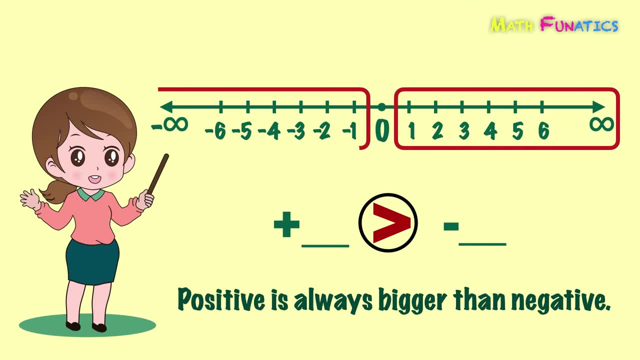 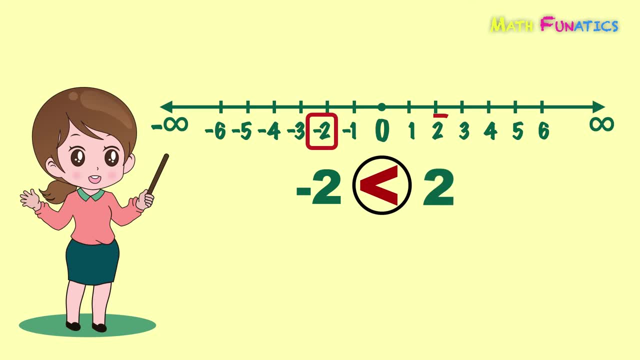 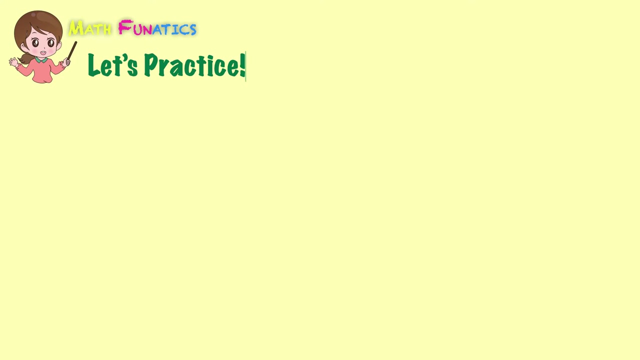 And all the negative numbers are on the left. So negative 2 is less than 2.. Negative 6 is less than 6.. Negative 100 is less than 100.. Now let's practice what you've learned about comparing integers. 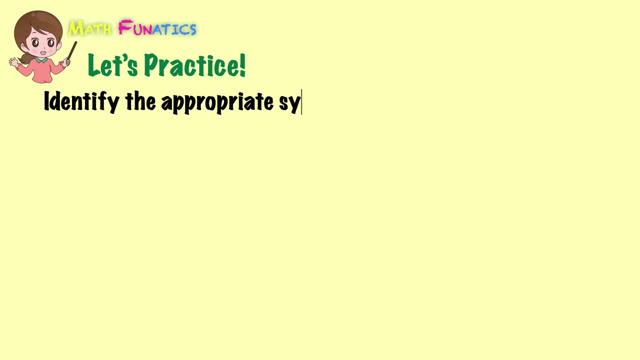 Identify the appropriate symbol for each comparison. The first is positive 18 and positive 11.. Since both are positive and 18 is on the right of 11 in the number line, then 18 is greater than 11.. Next we have positive 50 and 50.. 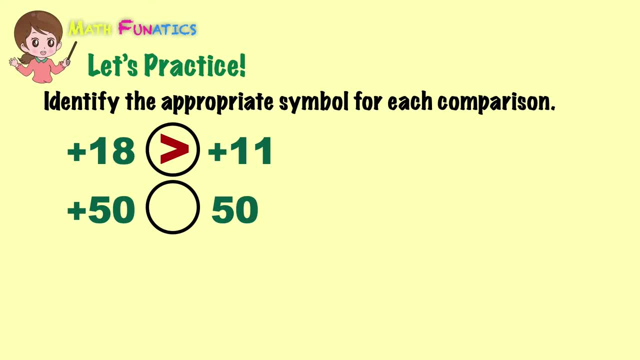 Both are actually positive 50, even though the second number has no sign. So they are equal: Negative 45 and negative 50, both are negative integers. Negative 45 is on the right of negative 54 and in fact nearer to zero. 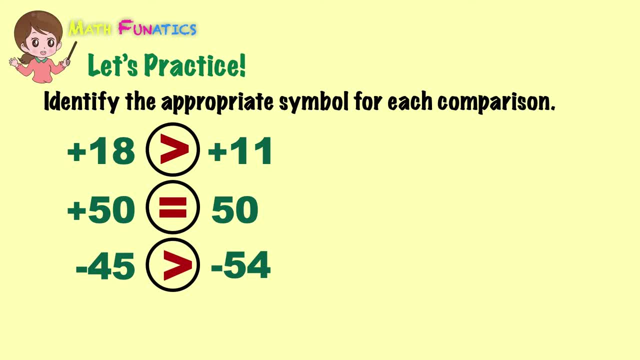 So negative 45 is greater than negative 54.. Negative 600 and negative 60. Negative 600 looks quite bigger than negative 60, but then it is actually found on the far left side of negative 60. So negative 600 is less than negative 60.. 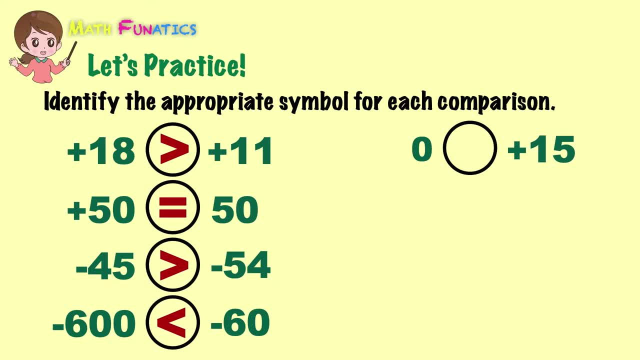 Zero and positive 15.. We've mentioned earlier that all positive numbers are greater than zero. So zero is less than 15.. Zero and negative 10. All negative numbers are less than zero, So we put here the greater than symbol. 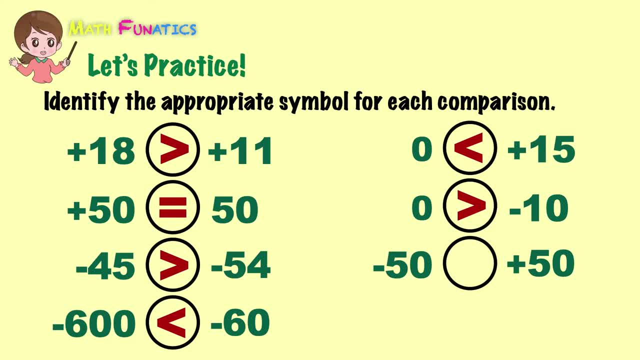 Negative 50 and positive 50. In this case, both are 50, but of different signs, Since negative integers are less than positive integers. therefore, negative 50 is less than positive 50.. Positive 10 and negative 100.. This last comparison applies, the one we mentioned in the previous question. 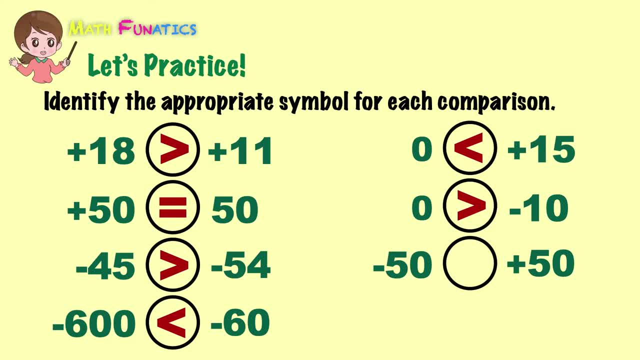 Negative 50 and positive 50. In this case, both are 50, but of different signs, Since negative integers are less than positive integers. therefore, negative 50 is less than positive 50.. Positive 10 and negative 100.. This last comparison applies, the one we mentioned in the previous question. 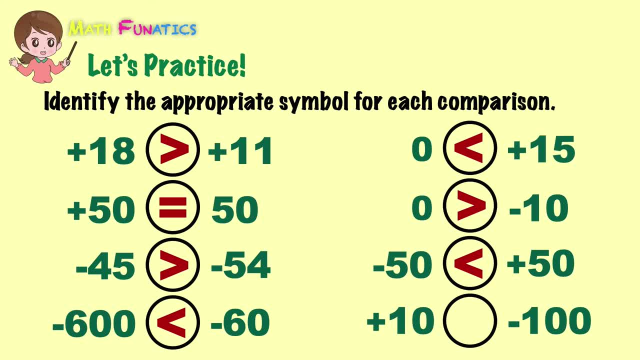 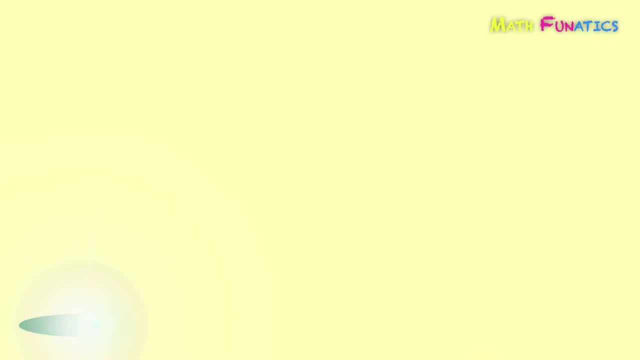 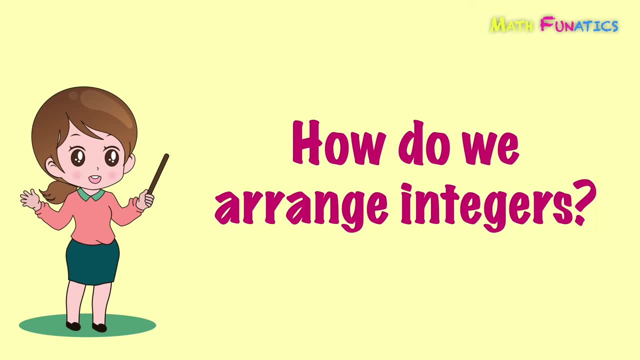 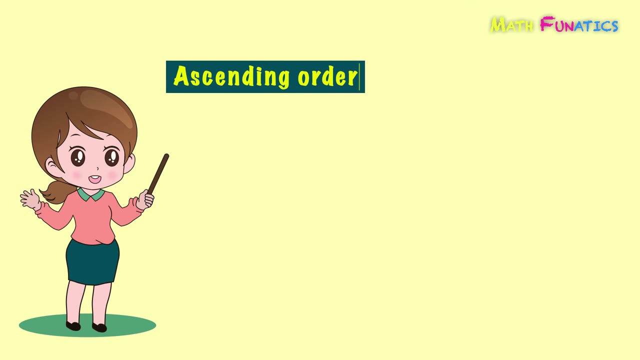 that negative numbers are less than positive numbers. So positive 10 is greater than negative 100.. This time, how are we going to arrange integers? We have two ways of arranging or ordering integers. First we have the ascending order. This is also called increasing order. 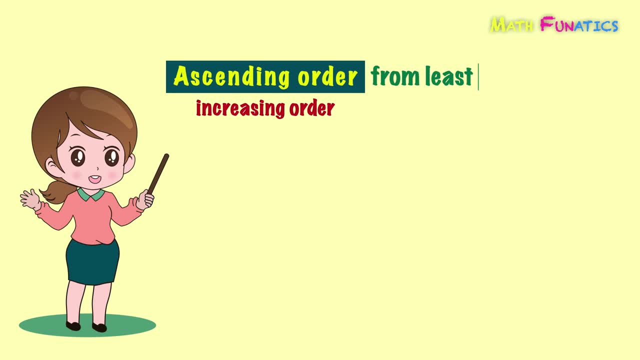 in which the integers are arranged for From least to greatest. The second one goes the opposite way: the descending order. This is also called the decreasing order, in which the integers are arranged from greatest to least. In ordering integers, same rules from comparing integers are applied. 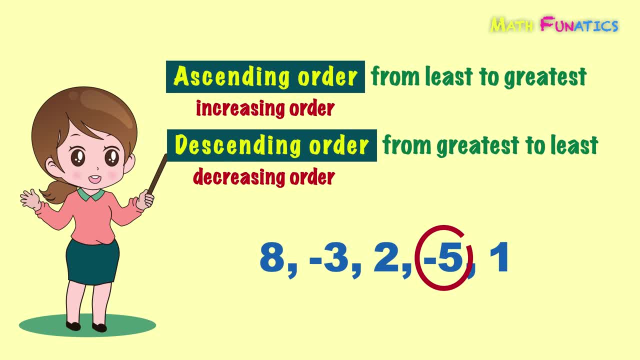 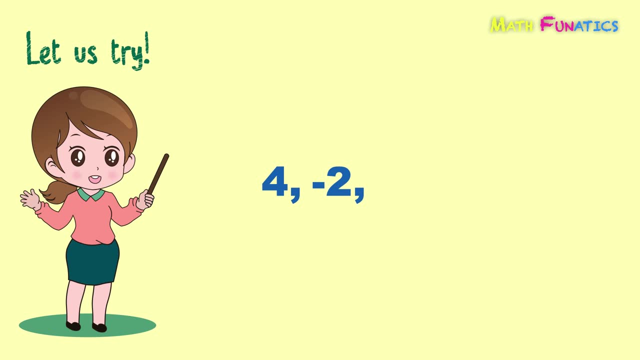 We just need to identify which among the given integers has the least value, the greatest value, and arrange them. Let's try doing it with these integers: Arrange positive 4, negative 2, positive 7, negative 1, and 0. 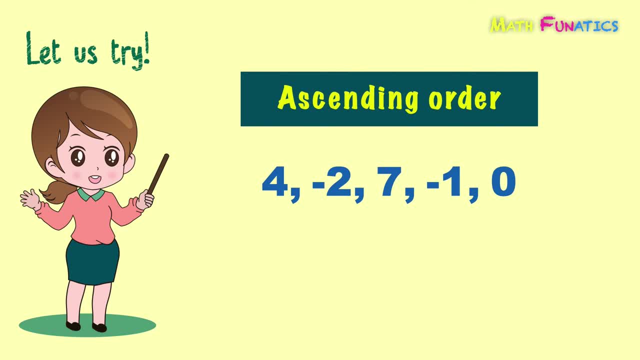 in ascending order. Remember that, in ascending order, the first integer that we have to write must be the one with the least value. Among these integers, negative 2 has the least value and negative 2 has the least value. Next is negative 1.. 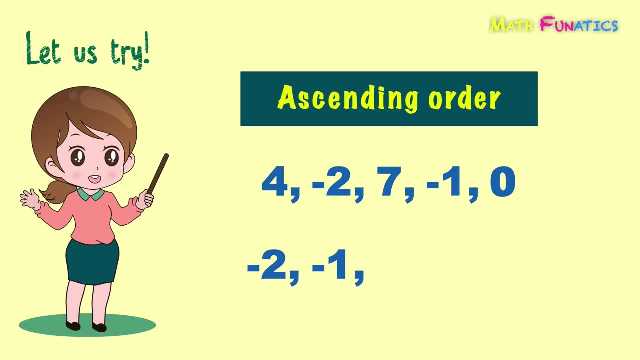 What comes next? Correct, It is 0. Then we write positive 4.. And the last is positive 7, since it is the integer with the greatest value. This time let's do the descending order with this set of integers: Negative 10,, positive 9,. 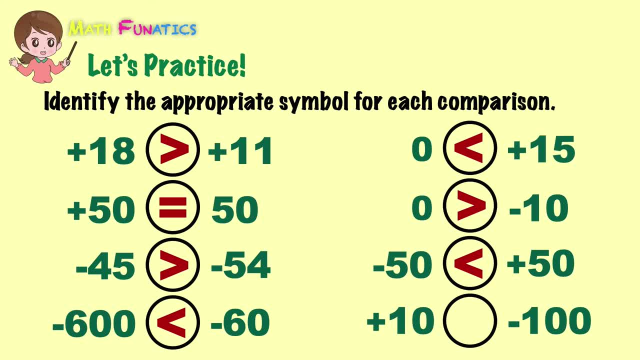 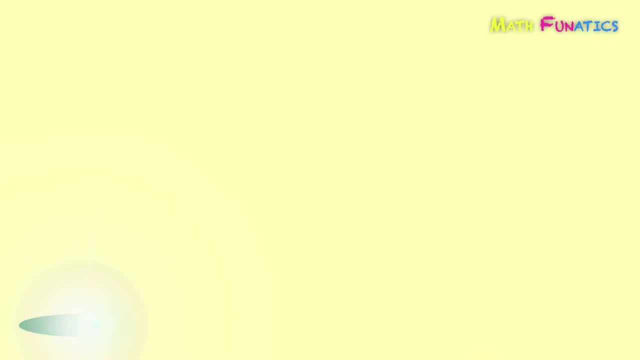 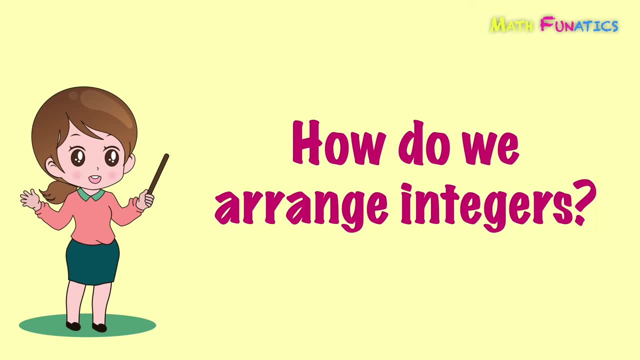 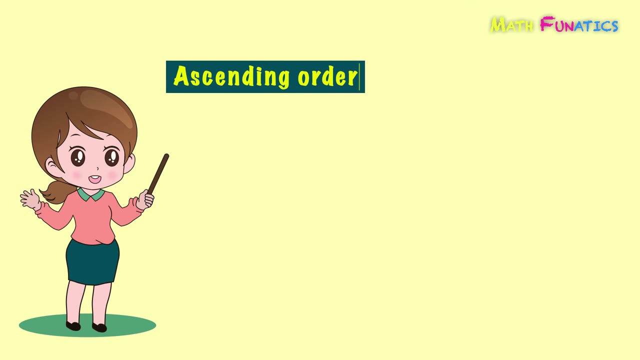 that negative numbers are less than positive numbers. So positive 10 is greater than negative 100.. This time, how are we going to arrange integers? We have two ways of arranging or ordering integers. First we have the ascending order. This is also called increasing order. 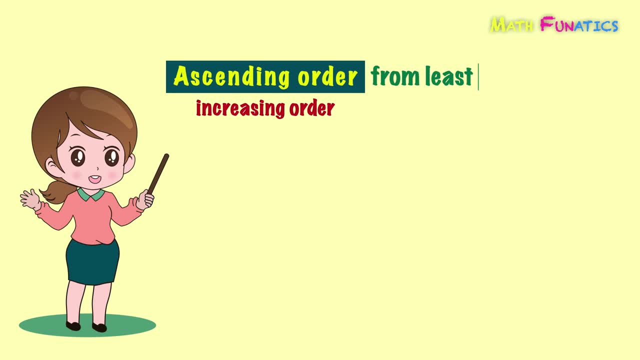 in which the integers are arranged for From least to greatest. The second one goes the opposite way: the descending order. This is also called the decreasing order, in which the integers are arranged from greatest to least. In ordering integers, same rules from comparing integers are applied. 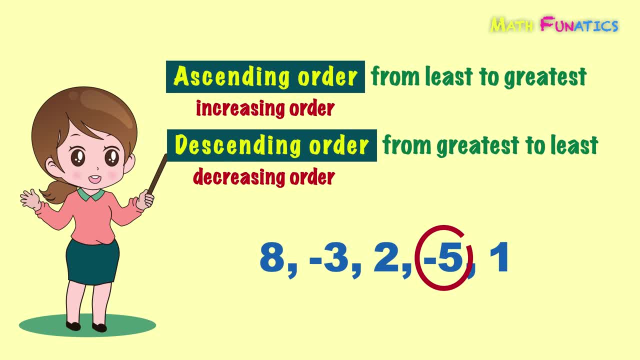 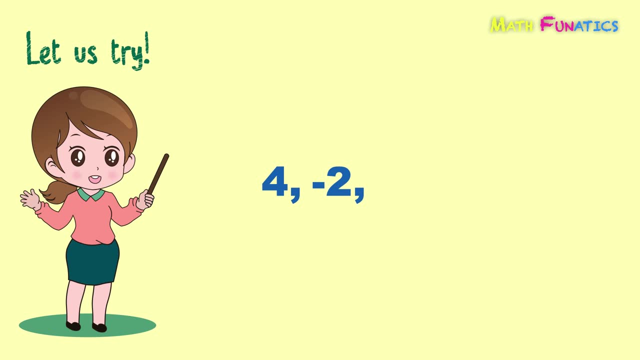 We just need to identify which among the given integers has the least value, the greatest value, and arrange them. Let's try doing it with these integers: Arrange positive 4, negative 2, positive 7, negative 1, and 0. 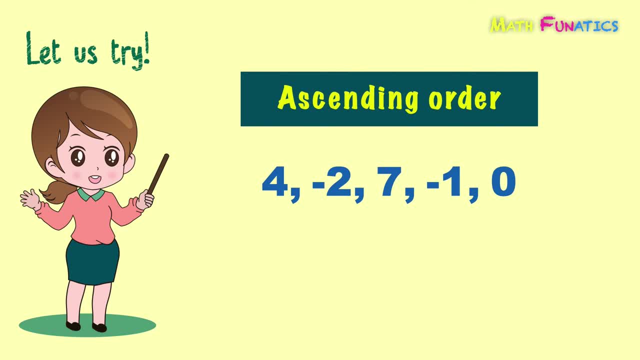 in ascending order. Remember that, in ascending order, the first integer that we have to write must be the one with the least value. Among these integers, negative 2 has the least value and negative 2 has the least value. Next is negative 1.. 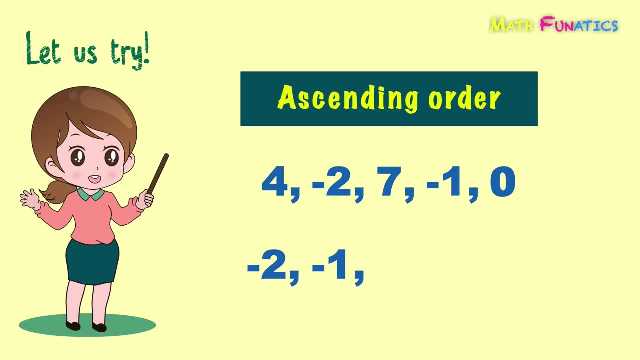 What comes next? Correct, It is 0. Then we write positive 4.. And the last is positive 7, since it is the integer with the greatest value. This time let's do the descending order with this set of integers: Negative 10,, positive 9,. 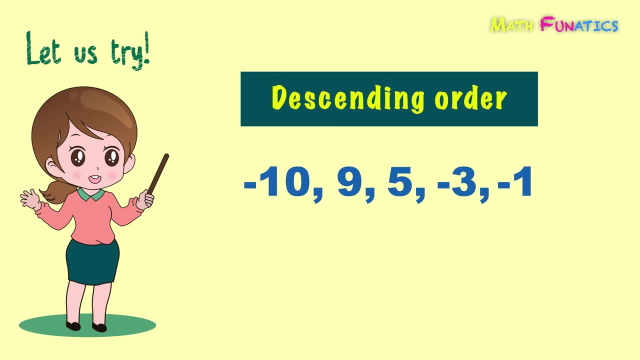 positive 5,, negative 3, and negative 1.. Take note that descending means decreasing, So we write first the integer with the greatest value, And it is positive 9, which must be written first, followed by positive 5.. Now, all the remaining integers are negative.